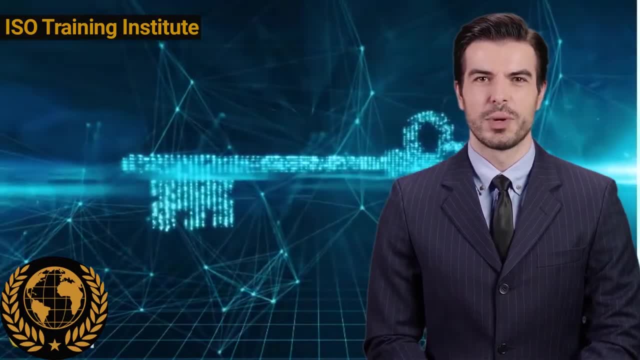 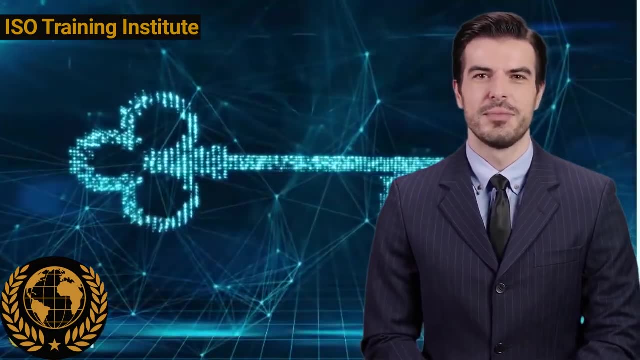 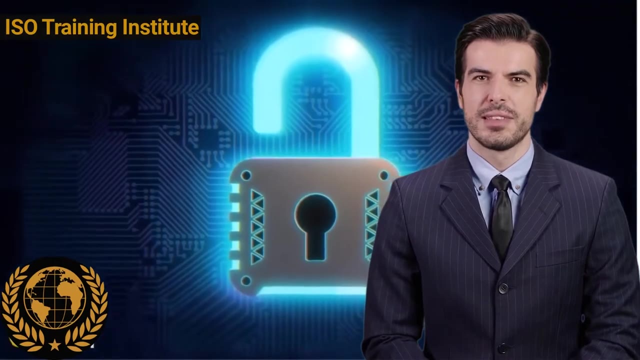 information security assessment. Otherwise it would be professional harakiri, Japanese term for ceremonial suicide. Here goes the high-level deep pointers: 1. What engineering-based security architecture solutions are considered at HLD and LLD on the basis of software's current requirement? 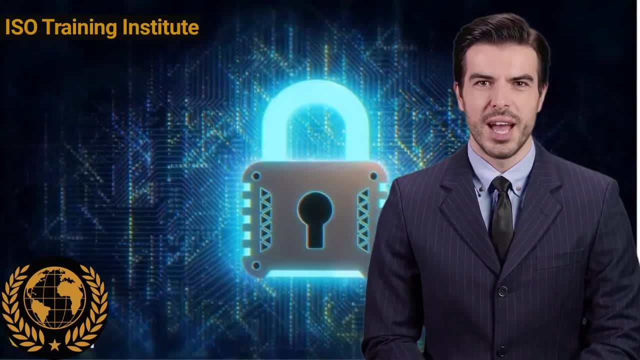 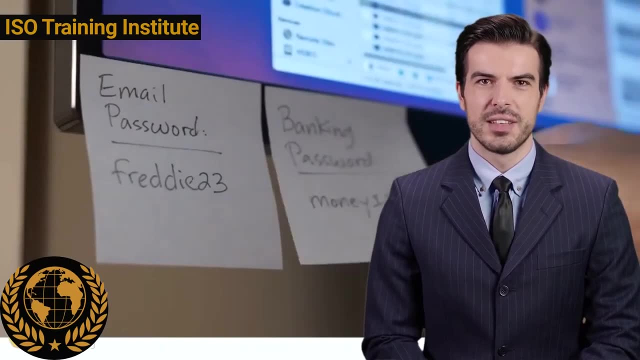 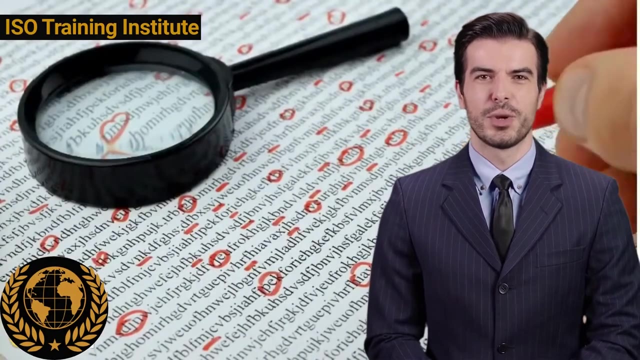 and future ramp-ups, including multitude of interfaces, add-ons and plugins. 2. How SDLC management system are ensuring that information at rest, information under process and information in transit remain confidential, remains available and integrity maintained in accordance with the information value and information exposure risk. 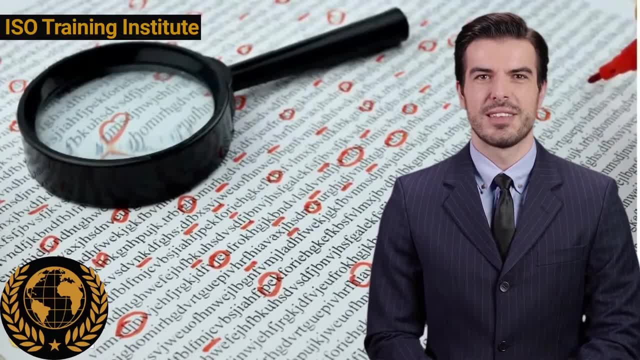 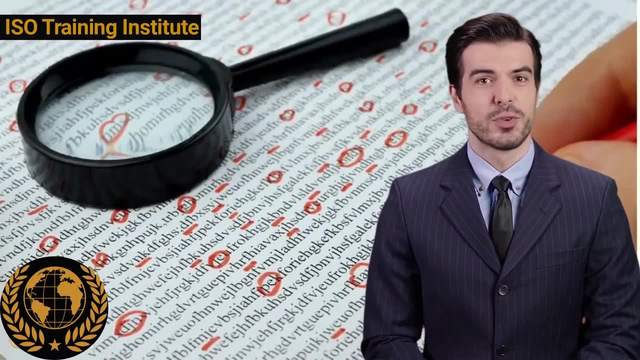 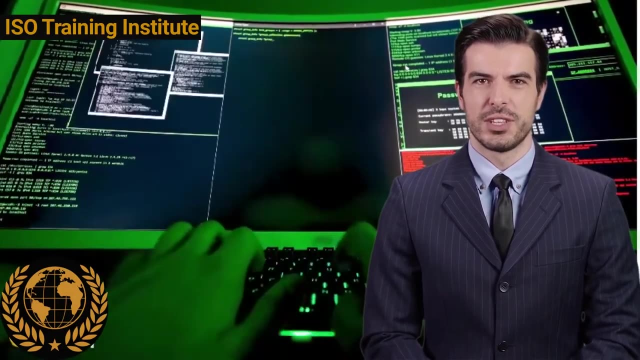 value. 3. How the SDLC processes are carried out on the basis of RBT- risk-based thinking. 4. What information security controls are in place triggered due to RBT. 5. What PDCA rigors are followed for the deployed information security controls. 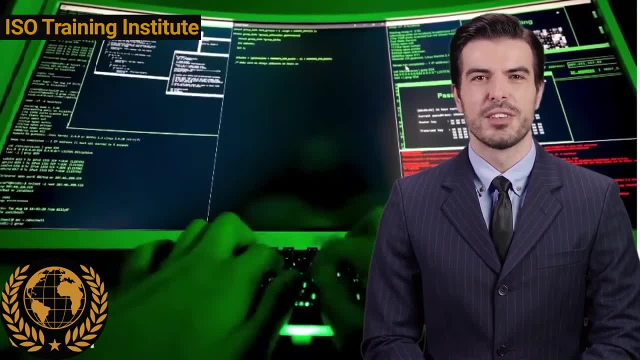 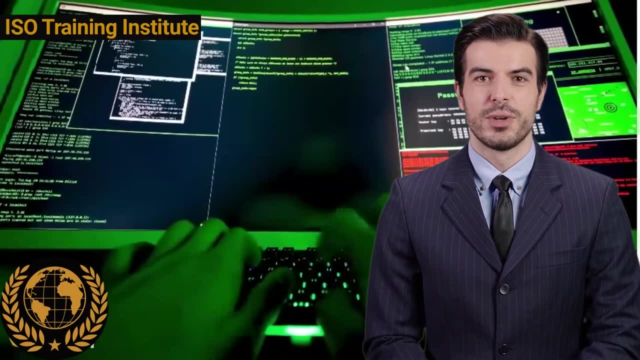 lifecycle management. 6. What are the strategy and metrics practices covering planning, security and risk management? 7. What are the strategy and metrics practices covering planning, assigning roles and responsibilities, identifying software security goals, determining budgets and identifying metrics and software release? 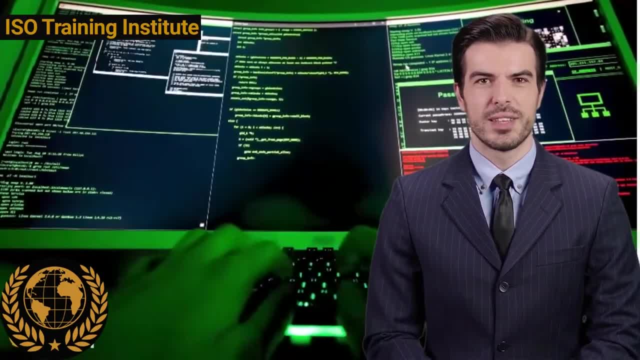 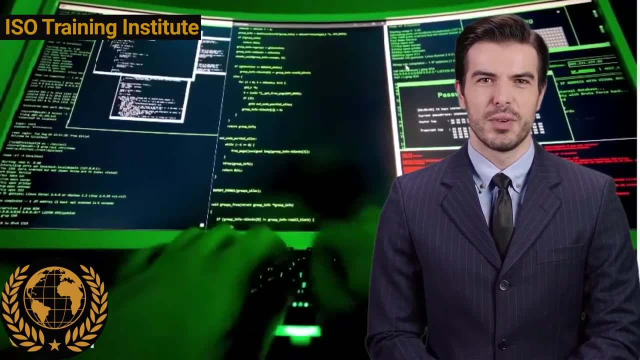 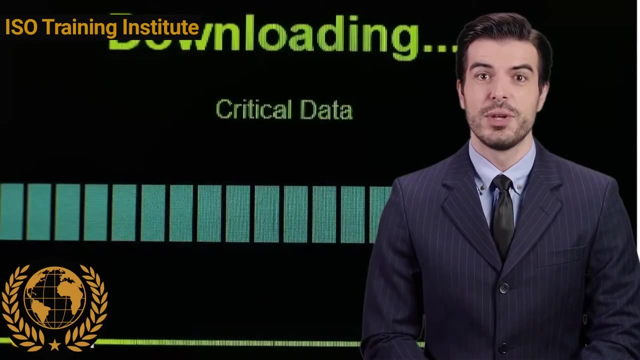 conditions. 7. How the compliance and policy practice focuses on identifying controls for compliance regimens such as HIPAA and PCI-DSS. build contractual SLA controls to enable COTS software risk controls. setting organizational software security policy and auditing against that policy. 8. What are the strategy and metrics practices? 7. What are the strategy and metrics? 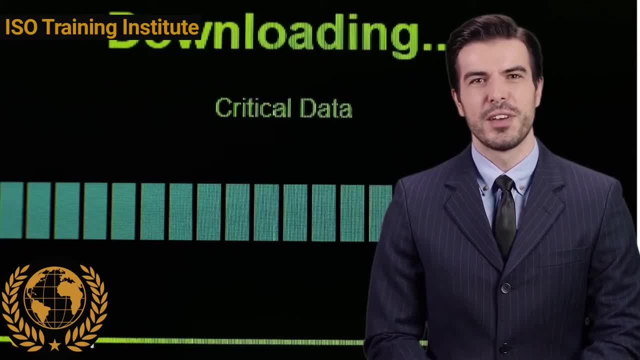 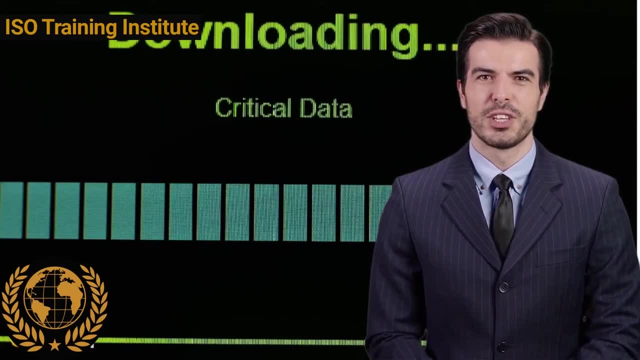 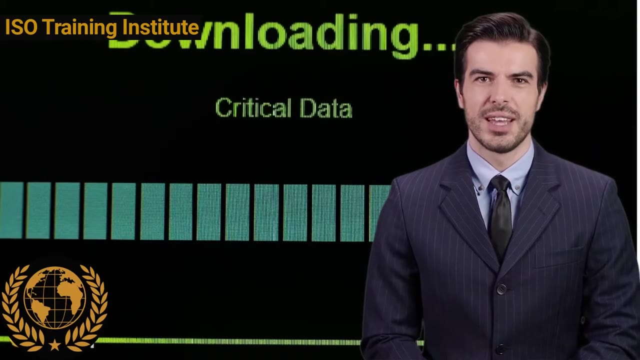 practices. 8. Show evidence of security-related training provided to architects, developers and testers. 9. Show evidence of attack models to capture information used to think like an attacker: threat modeling, abuse case development and refinement, data classification and technology-specific attack patterns. 10. Rather than having each project team implement, 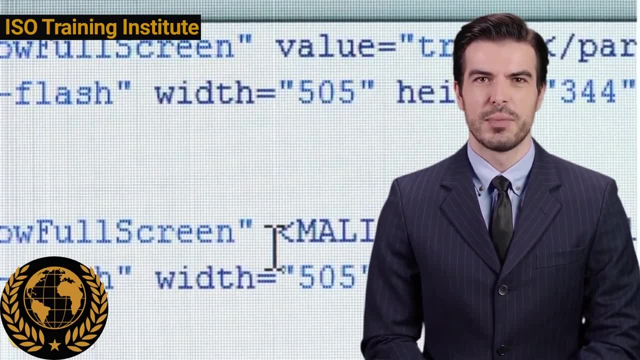 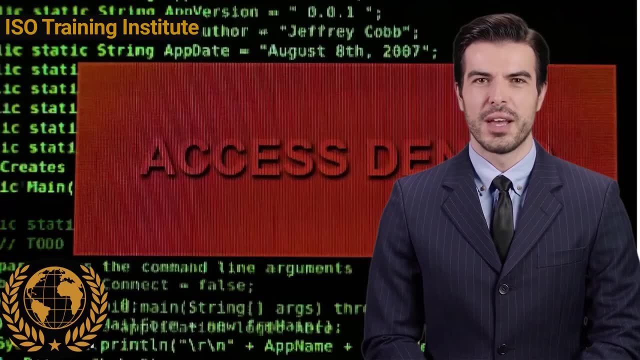 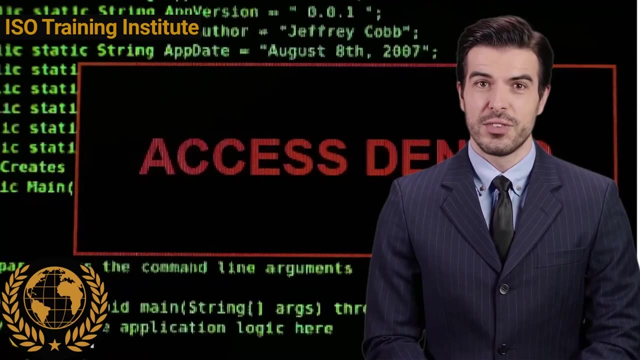 its own security features, such as authentication, role management, key management, logging, cryptography protocols. show evidence that the software security group SSG provides proactive guidance by acting as or facilitating a clearinghouse of security features for engineering groups to use. 11. Show evidence of architecture analysis covering software architecture in 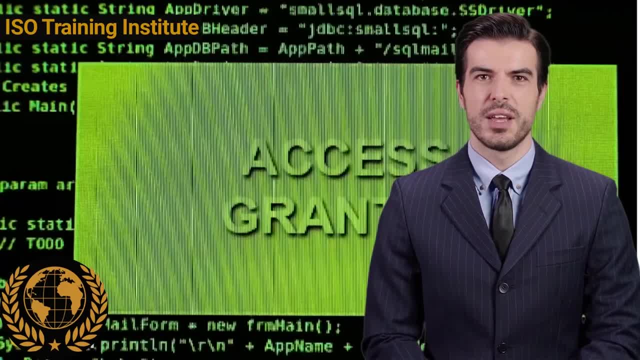 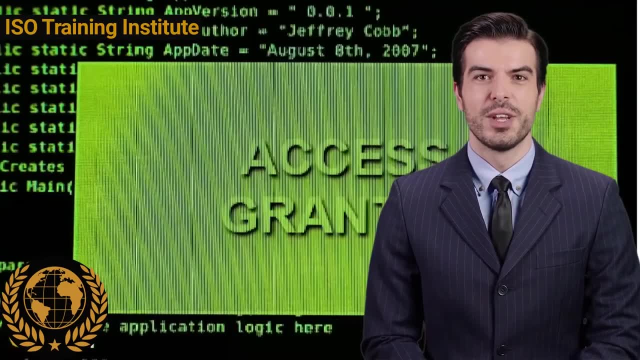 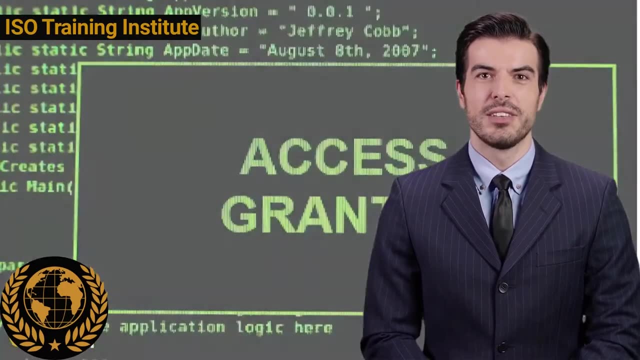 concise diagrams, applying lists of risks and threats, adopting a process for review, such as architecture risk analysis, and building an assessment and remediation plan for the organization. 12. The security testing practice is concerned with pre-release testing, including integrating security into standard quality assurance processes. 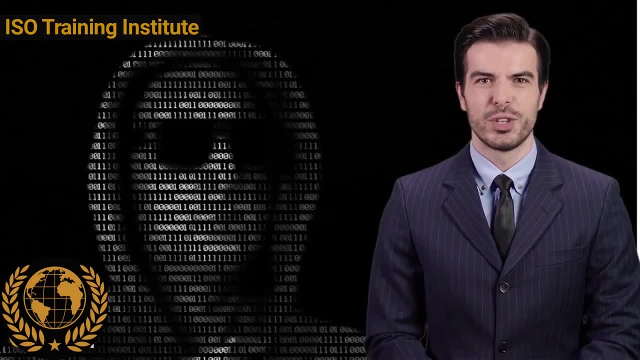 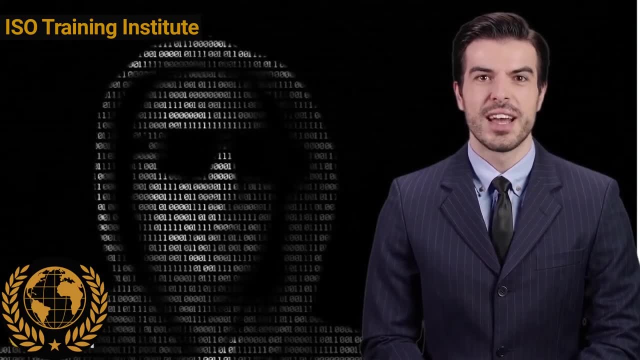 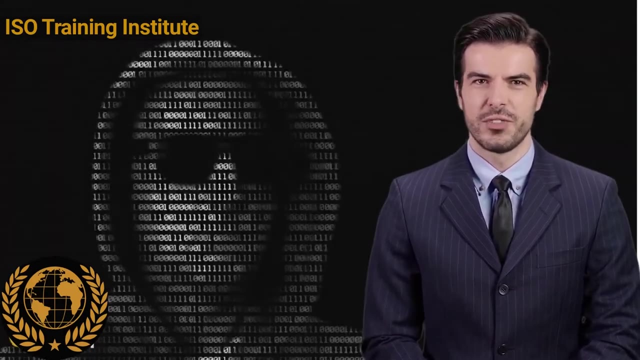 Show evidence that the practice includes use of black box security tools, including fuzz testing as a smoke test in QA, risk-driven white box testing, application of the attack model and code coverage analysis. 13. How do you capitalize the penetration testing practice involving standard outside and testing of the sort carried out? 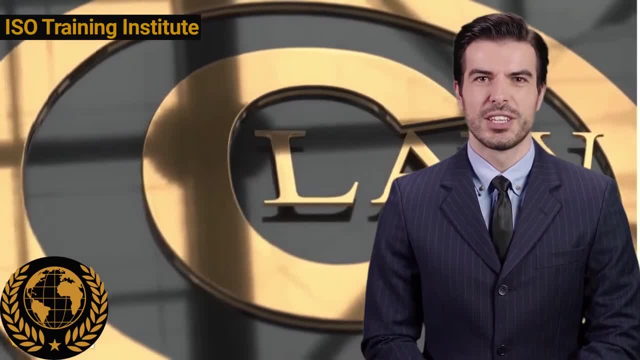 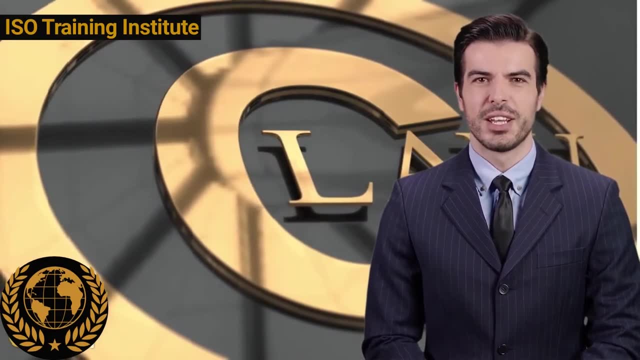 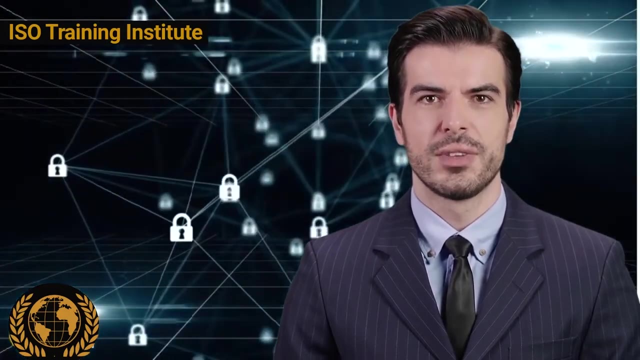 by security specialists. Show evidence of how penetration testing dredges out vulnerabilities in the final configuration and provides direct feeds to defect management and mitigation. 14. Show evidence of the software environment practices that deal with OS and platform patching, including in the cloud WAFS installation and configuration documentation. 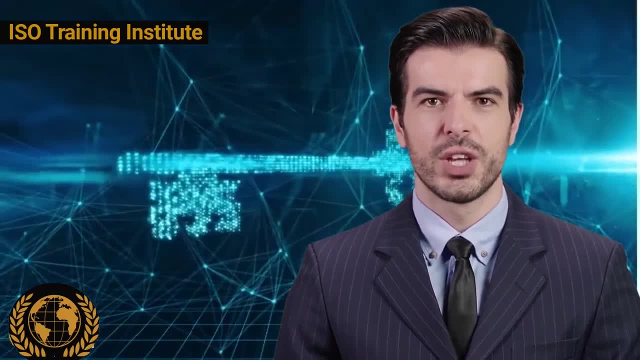 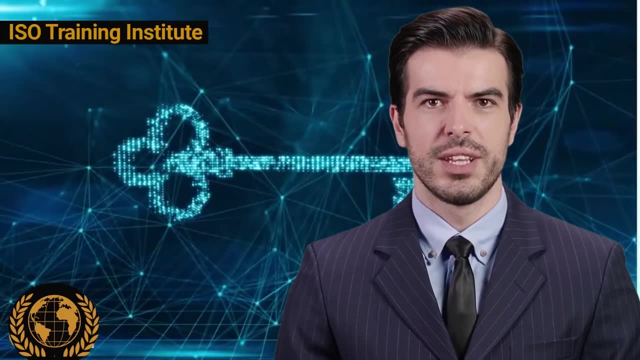 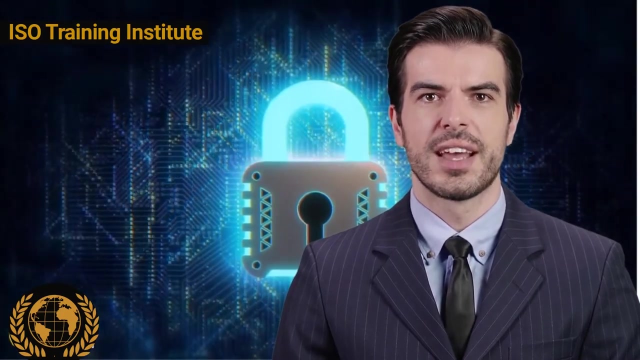 containerization, orchestration, application monitoring, change management and code science. 15. Show evidence of how the configuration management and vulnerability management practice concerns itself with patching and updating applications, version control, defect tracking and remediation and incident handling. 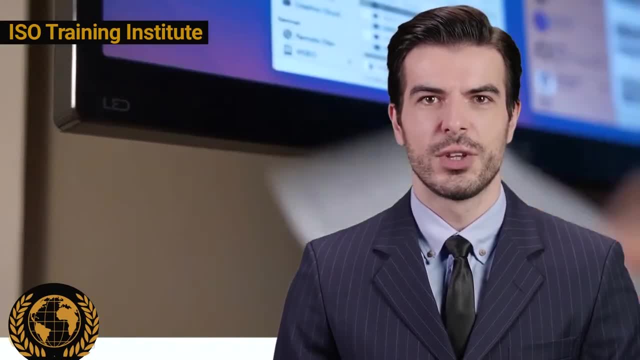 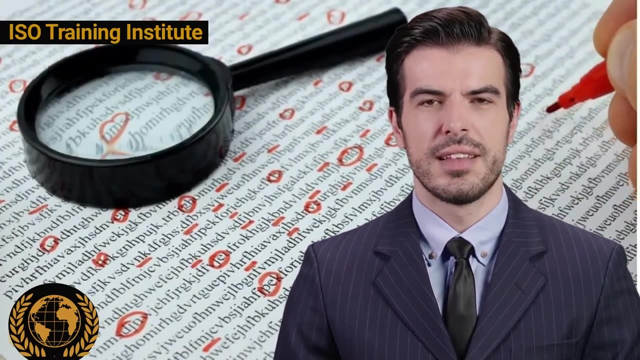 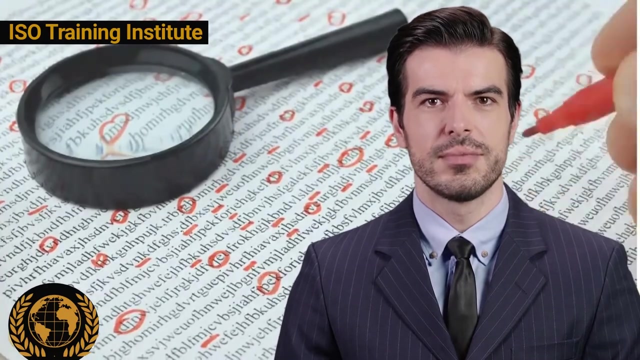 These are the trivia or most simple SDLC security tip of the iceberg: compliance questionnaires that need to be asked from the department during audit. At best you can call them warm-up questions prior to start of the decathlon compliance audit on SDLC security. The colossal damages in terms of cost implications and careers disruptions. 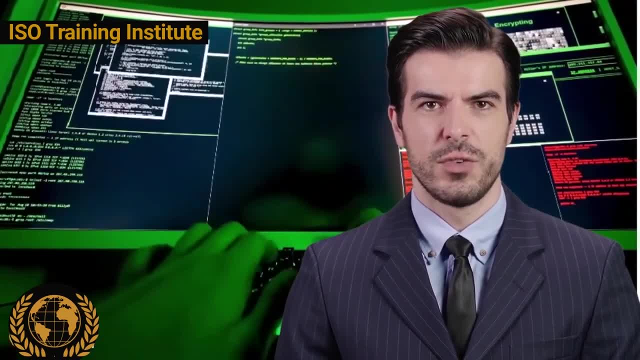 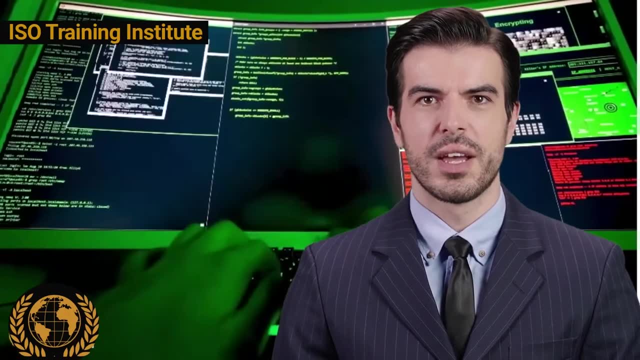 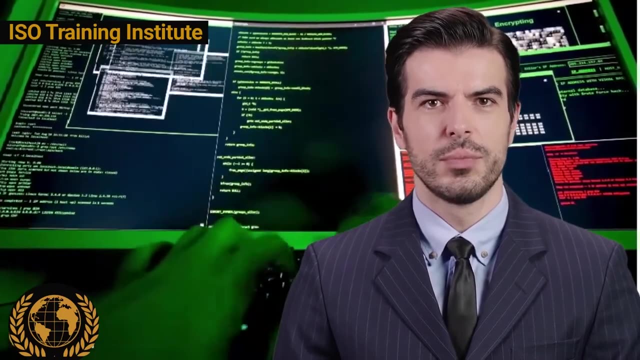 caused by these SDLC security breaches are avoidable, provided the companies and the professionals responsible for managing the information security are not complacent and do not get certifications for ornamental purpose alone. There is popular misnomer that SDLC security breach, just like death happens to somebody else, until your time runneth over. 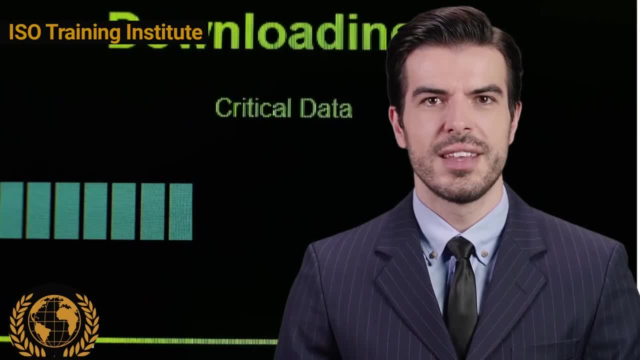 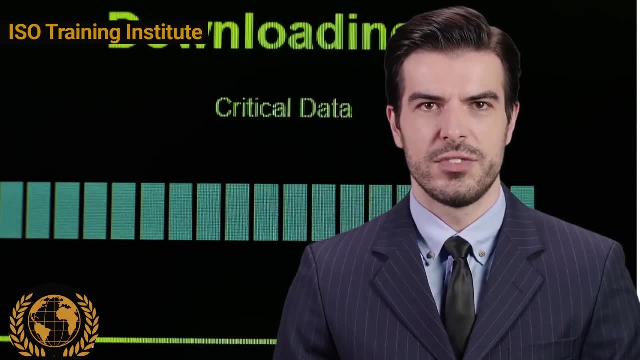 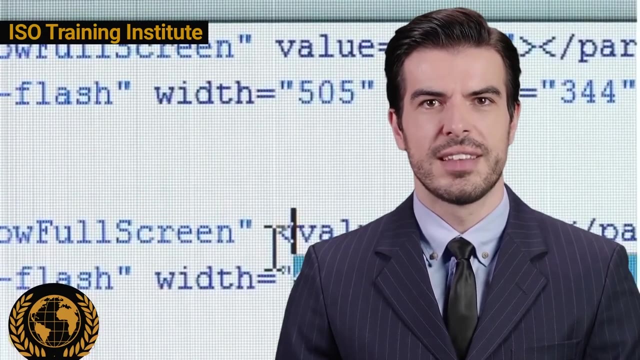 SDLC security checklists in accordance with ISO 27001, having more than 315 compliance questions has been prepared by the collective wisdom of panel of information security principal auditors and lead instructors under the aegis of ISO Training Institute. Lots of effort has gone into preparing it and making it available. It does not include website. 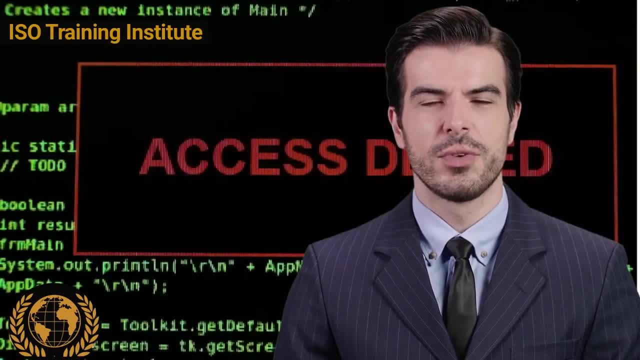 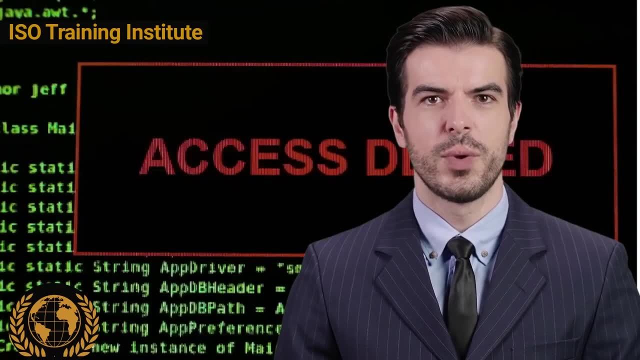 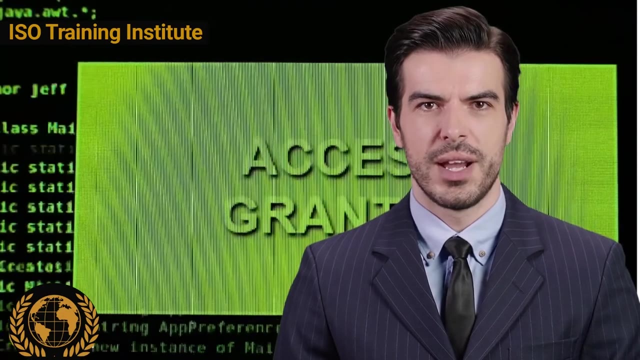 security and application security. because of enormity of unique security compliances, These have been used to prepare for and maintain compliance questions. These have been made available separately. These comprehensive, deep-probing, robust checklists are unparalleled in the entire world. The SDLC security checklists have been prepared. 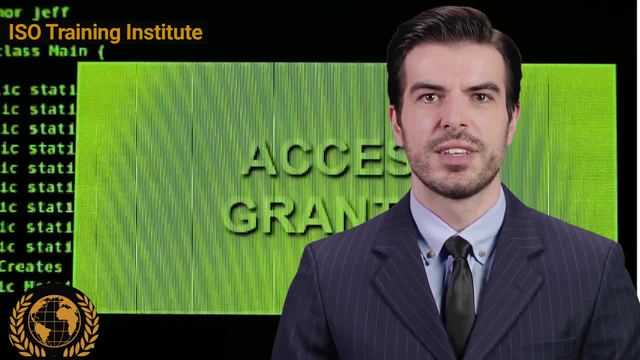 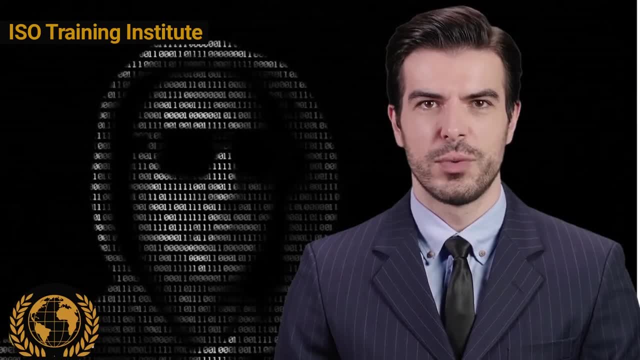 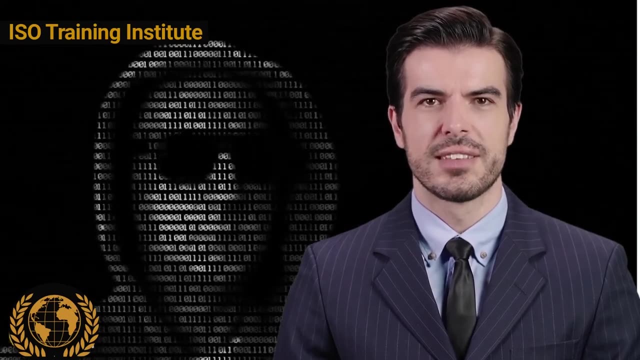 with a noble spirit of reducing these colossal damages to the organizations and professional careers, including yours. You have a choice: to be continued to remain vulnerable as the hunted by the security breaches which are the hunters, or proactively identify and neutralize them. 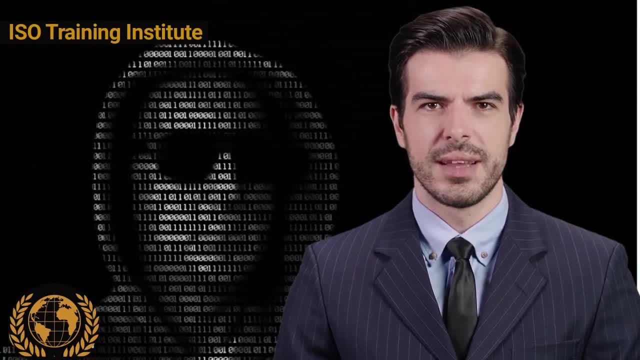 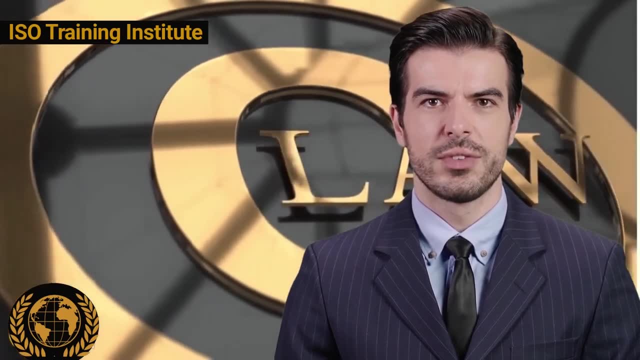 with the help of these robust compliance checklists. It is a choice between corporate longevity and corporate mortality. It is choice of not becoming scapegoat and protecting your careers and growth that you truly deserve. 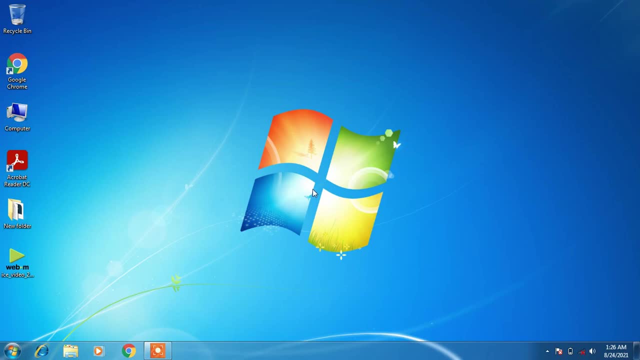 Hello everyone, I Vatsal, welcome you all to my channel and today I am going to show you how to fix the issue of Wi-Fi networks not showing in Windows 7.. So if you go to the taskbar over this network icon, you can clearly see that it is not showing the Wi-Fi networks. 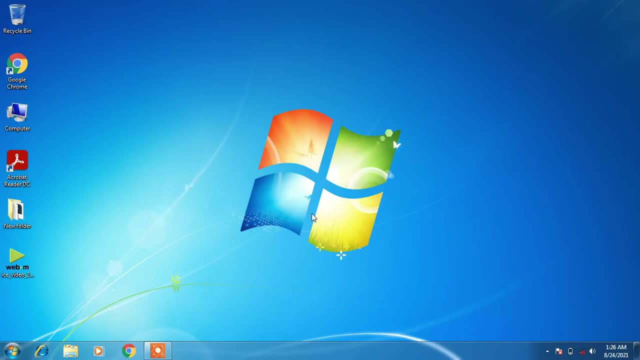 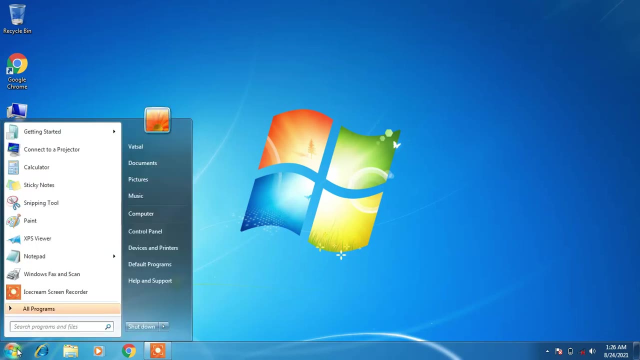 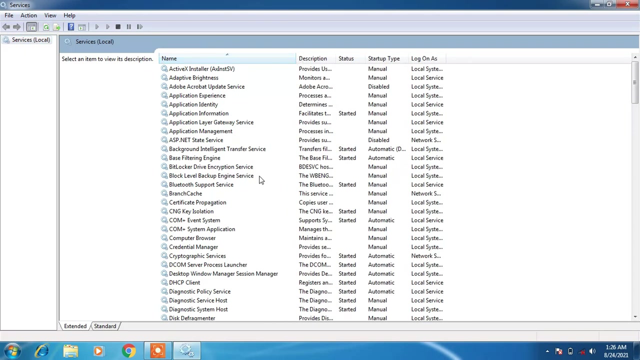 and I am not connected to the internet also. So if you are also facing the same issue, then there are three methods to fix this issue. Method number one is: just click on the start button, go to the search bar and type services. Now just click on the search result: services. 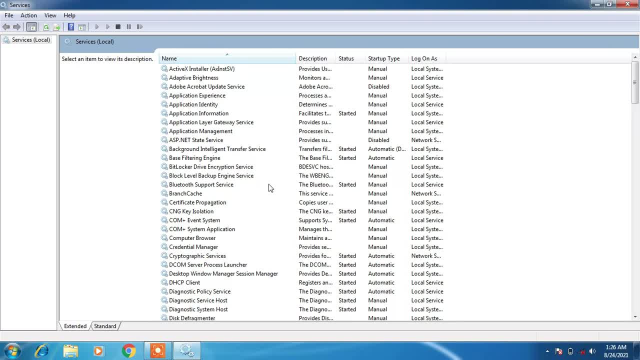 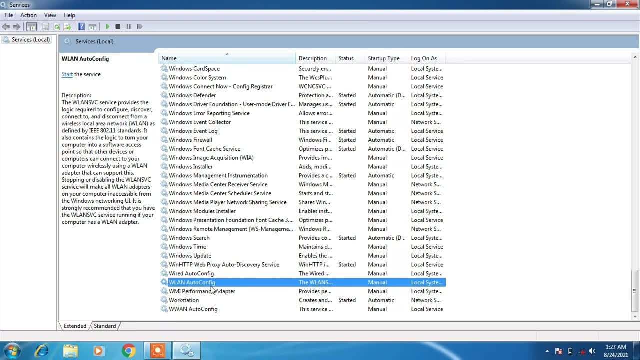 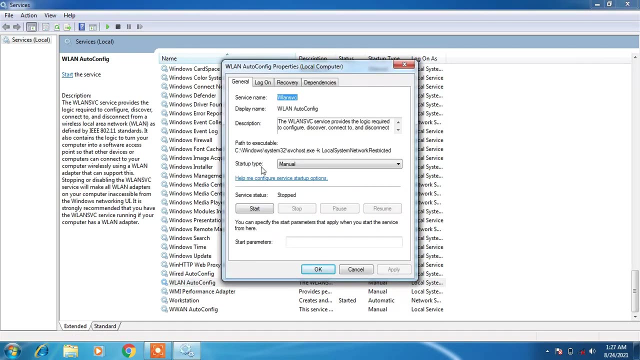 and now in this list of services, just search for WLAN auto-config. So here it is: WLAN auto-config. just right click over it and click on properties. Now just change the startup type from manual to automatic. After this, just click on the apply button. Then just click on the start button to start the service. After this, just